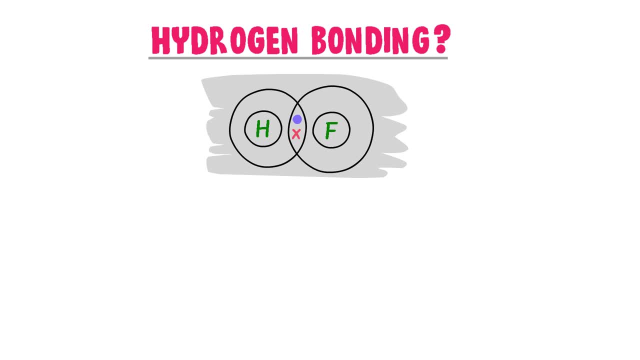 We know that hydrogen and fluorine atoms are chemically combined. due to covalent bond, Hydrogen and fluorine atoms mutually share one pair of electrons and form a single molecule of hydrogen fluoride. In this molecule, fluorine is highly electronegative than hydrogen. The 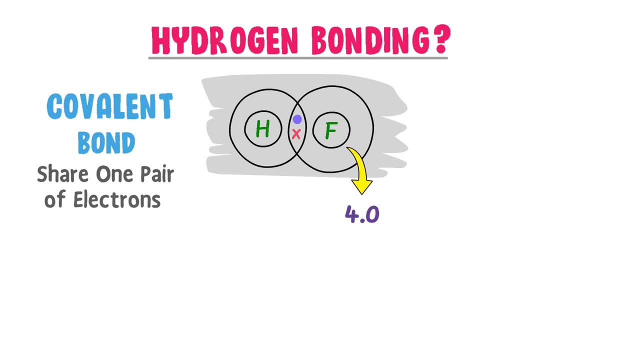 electronegativity of fluorine is 4.0 and the electronegativity of hydrogen is 2.1.. When we calculate the electronegativity of fluorine, the electronegativity of hydrogen is 2.1.. 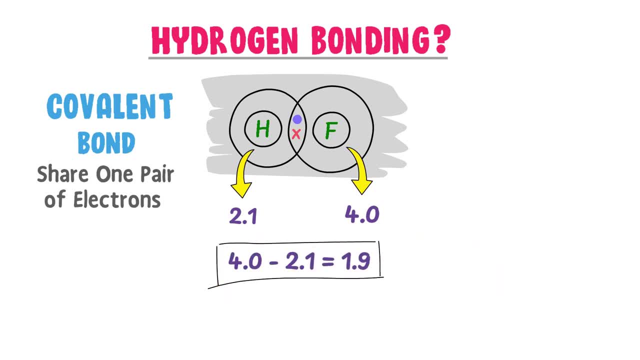 When we calculate the electronegativity difference of hydrogen fluoride, we get 1.9.. This is a very large difference in electronegativity. As a result of this fluorine atom, being highly electronegative, pulls the. 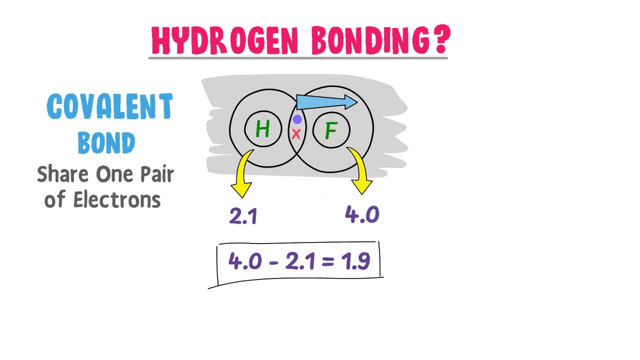 shared pair of electrons more towards itself than hydrogen. The electronic cloud tilts towards fluorine atom and partially negative charge appears on fluorine and partially positive charge appears on hydrogen. So therefore we say that hydrogen fluoride is a highly polarized molecule. 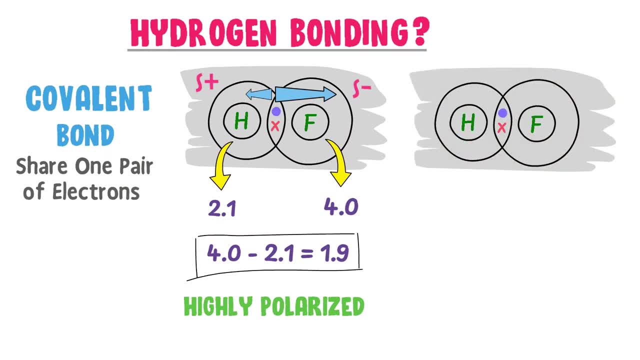 Now consider another molecule of hydrogen fluoride. Like this molecule, it also has partially negative pole and positive pole. Here there are two highly polarized molecules. Now listen carefully. The negative pole of this hydrogen fluoride molecule attracts the positive pole of this hydrogen fluoride molecule, The negative pole of this hydrogen fluoride molecule. 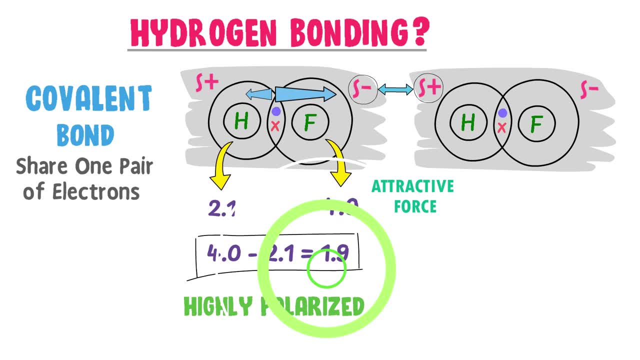 attracts the positive pole of this hydrogen fluoride molecule and the attractive force produces between them. Let me repeat it: The negative pole of this hydrogen fluoride molecule attracts the positive pole of this hydrogen fluoride molecule and the attractive force produces between them. This attractive force between these two molecules is called hydrogen. 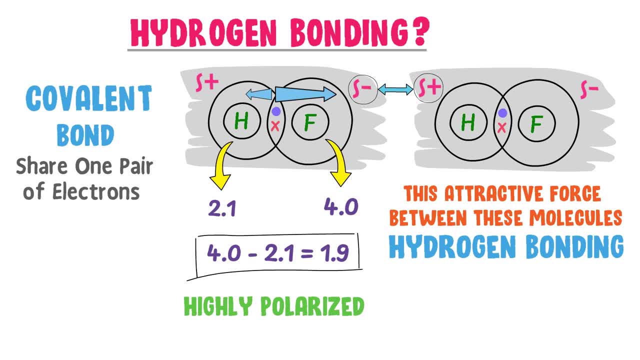 bonding. So hydrogen bonding is not a chemical bond. Rather it is intermolecular forces between molecules. The word inter means between. Thus hydrogen bonding is an attractive force between molecules. Also, remember that covalent bonding is an intramolecular force. The word 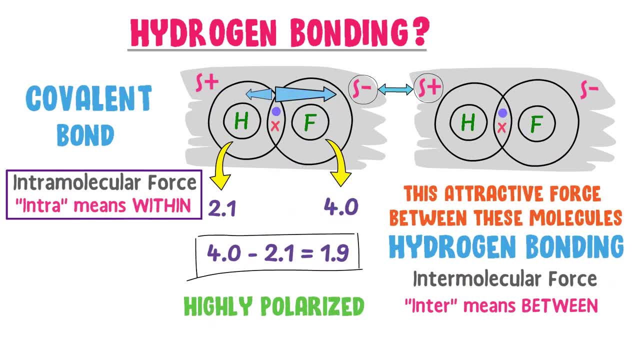 intra means within. So covalent bonding is a force within atoms. Therefore, remember that hydrogen bonding is the attractive force, or intermolecular forces between highly polarized molecules like hydrogen fluoride. Now let me ask you: Does hydrogen bond exist? 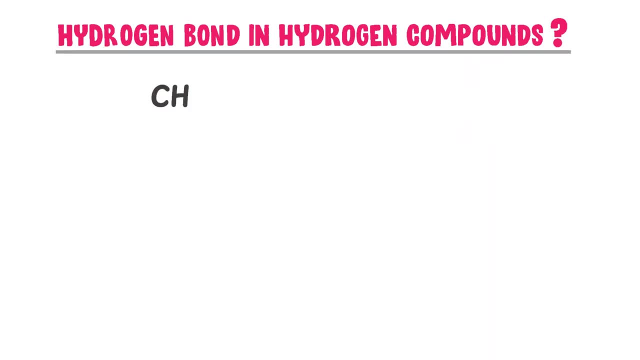 in all hydrogen compounds like methane, ethane and propane? Well, the answer is absolute: no. Hydrogen bond doesn't exist in these compounds because carbon is less electronegative. For instance, let we should calculate the polarity of carbon and hydrogen bond: The 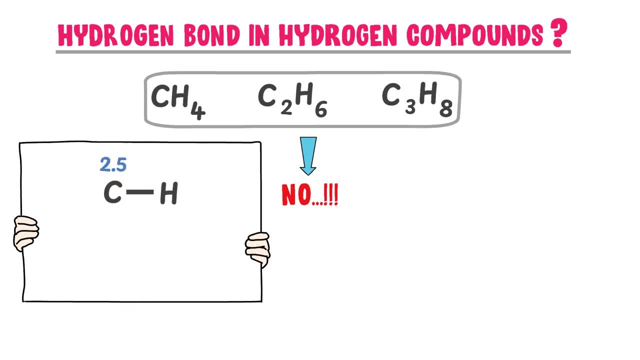 negativity of carbon is 2.5 and the electronegativity of hydrogen atom is 2.1.. When we calculate the electronegativity difference between these two atoms, we get 0.4.. It is very small difference. The bond between carbon and hydrogen is non-polar. So all these molecules are non-polar and 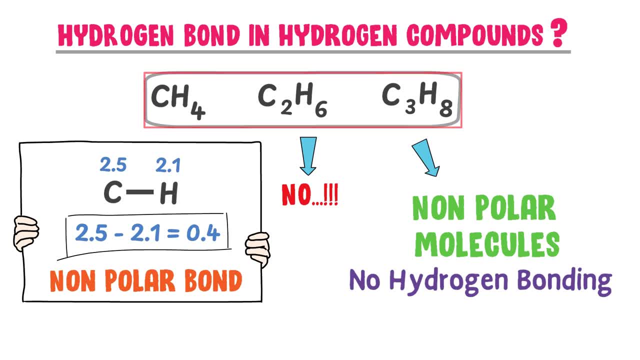 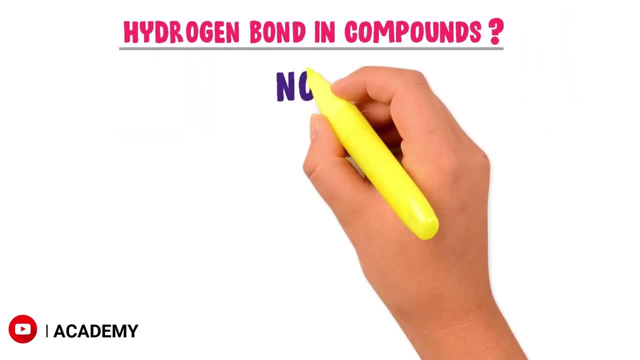 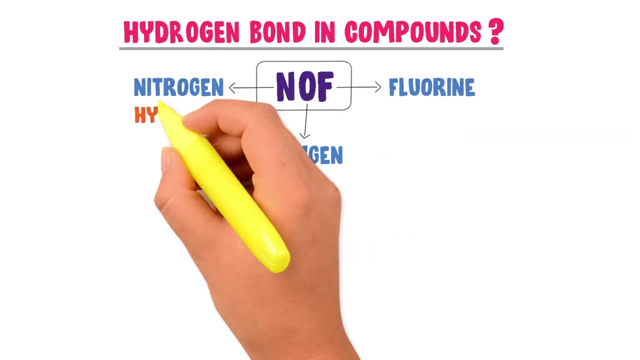 hydrogen bond doesn't exist in these compounds. Now, what are the compounds and what are the factors in which hydrogen bond exists? Well, remember this mnemonic NOF: I mean nitrogen, oxygen and fluorine, When hydrogen forms a covalent bond with these three elements. 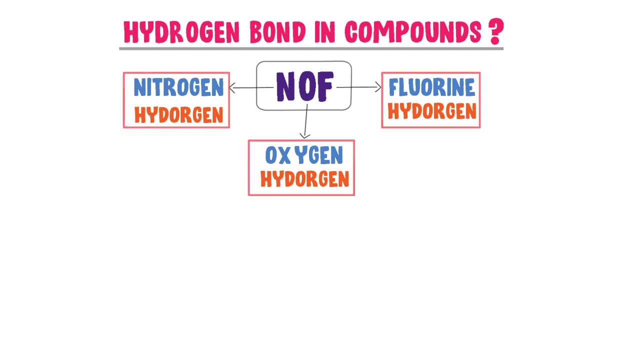 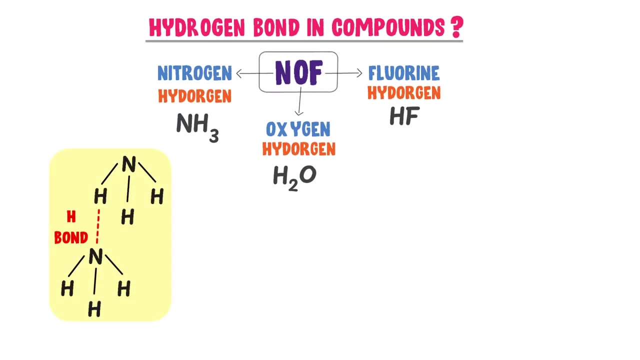 hydrogen bond exists between their respective molecules. For example, hydrogen bond exists in ammonia, water and hydrogen fluoride. Hydrogen bond exists between molecules of ammonia. hydrogen bond exists between molecules of water and hydrogen bond exists between molecules of hydrogen fluoride. Thus, note it down this mnemonic enough, and remember that hydrogen bond only exists in. 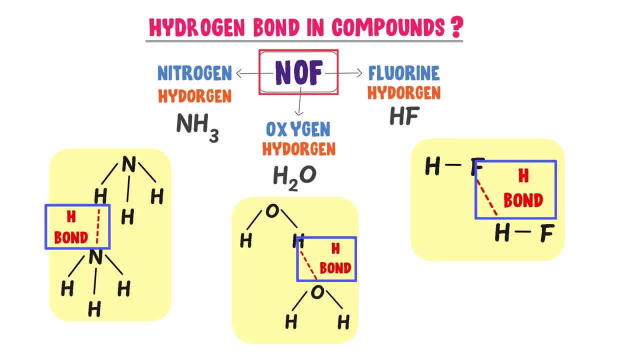 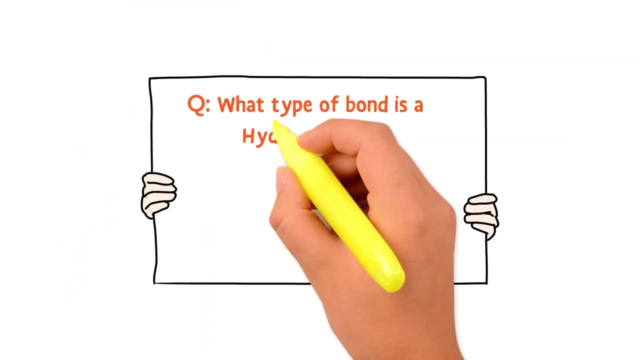 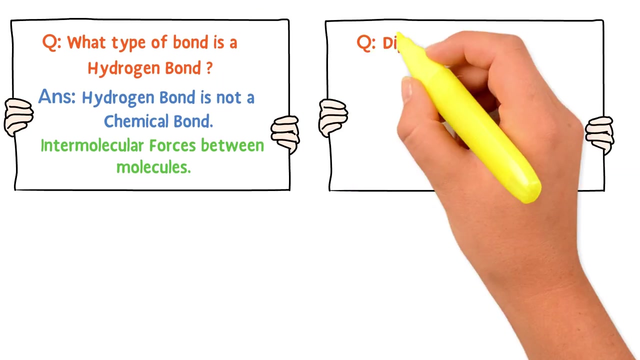 ammonia, water and hydrogen fluoride. Now let me teach you some bullet questions regarding hydrogen bonding. What type of bond is a hydrogen bond? Remember that hydrogen bond is not a chemical bond. Hydrogen bond is intermolecular forces between molecules. Secondly, which is stronger, dipole-dipole forces or hydrogen bonding?